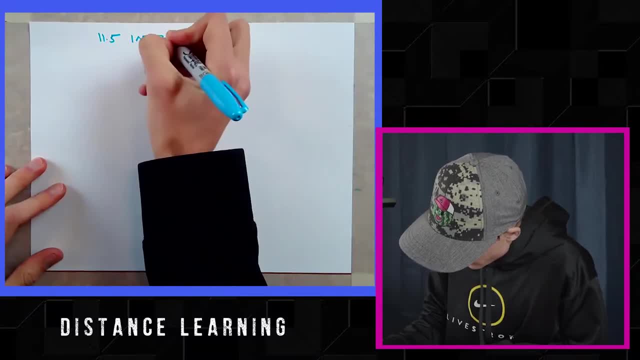 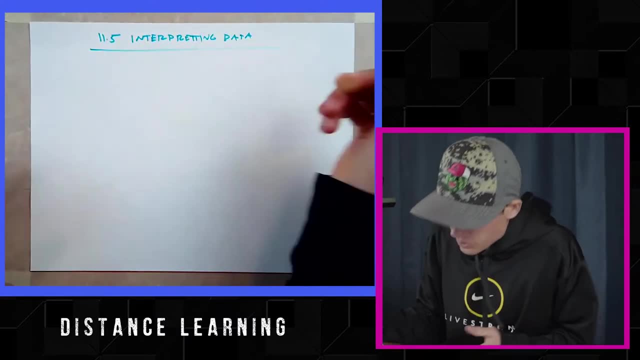 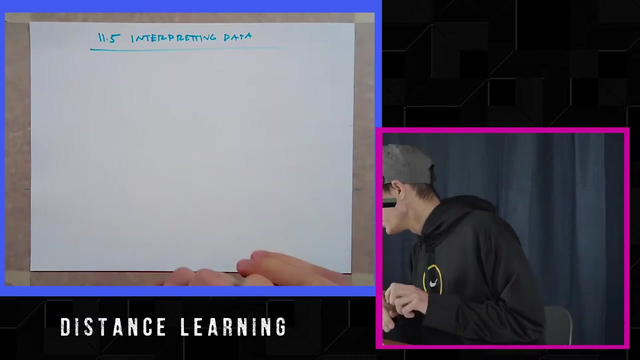 Interpreting data. Interpreting data And basically, after you've taken the surveys like you did, like you created in the last lesson, now you've got to interpret the data from said surveys. So they give you some TV thing. It says uh, 5,000.. 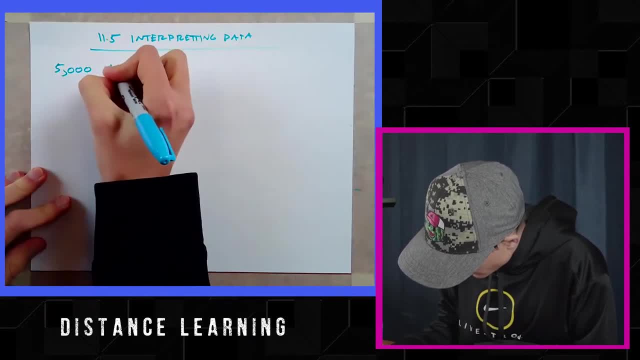 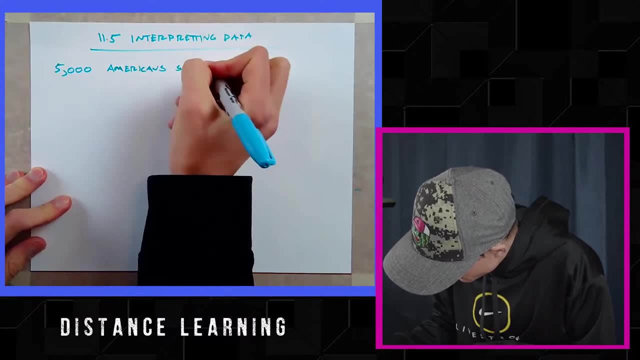 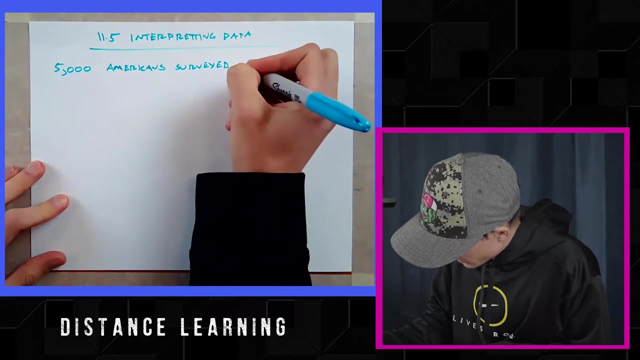 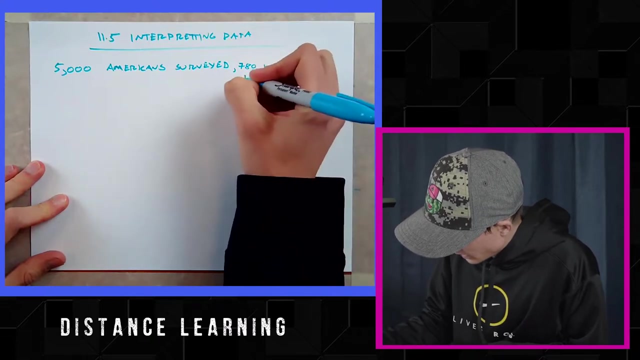 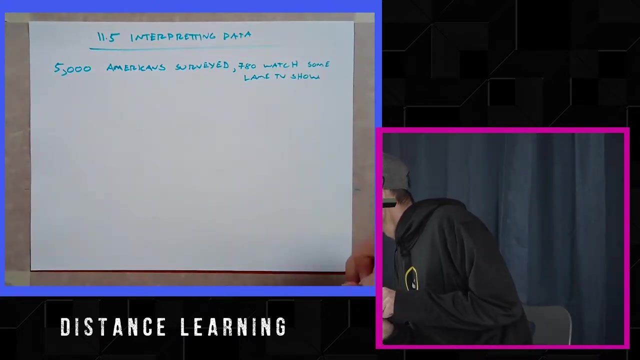 5,000 Americans surveyed. Wow, that's a good M Americans surveyed. 780 of them watch some lame TV show. Okay, So what they want you to do is: this was just a survey, right? There's more than 5,000 people in the United States. 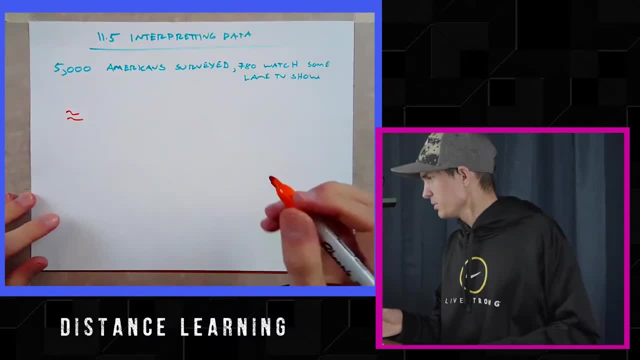 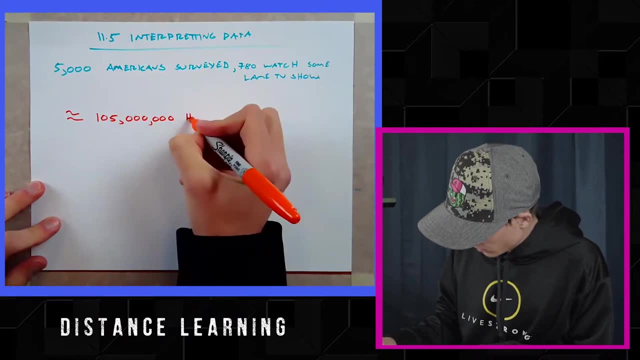 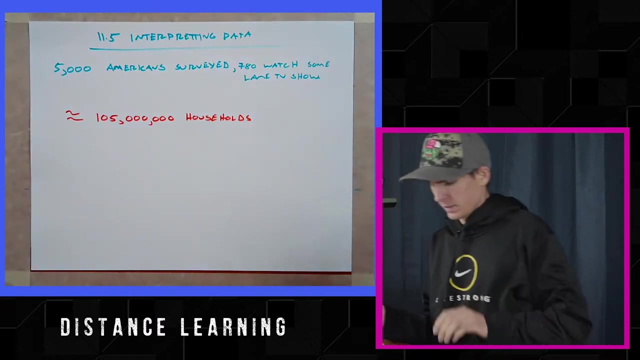 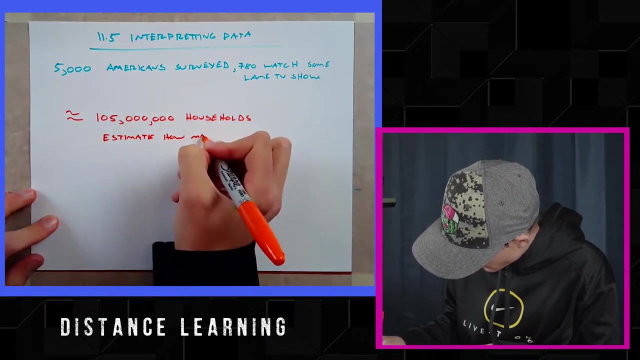 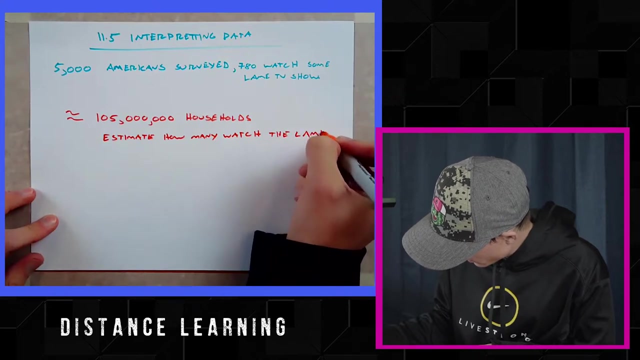 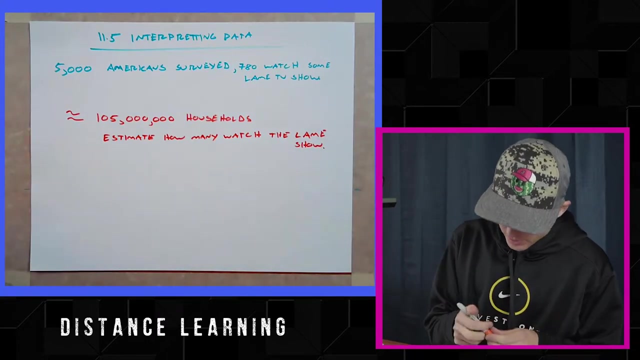 So there's, according to the book, at this time in the United States 105 million households In the United States- Not people, but households- And they want you to estimate how many watch the lame show. So normally when you do a survey, it could be that you actually ask everybody, right. 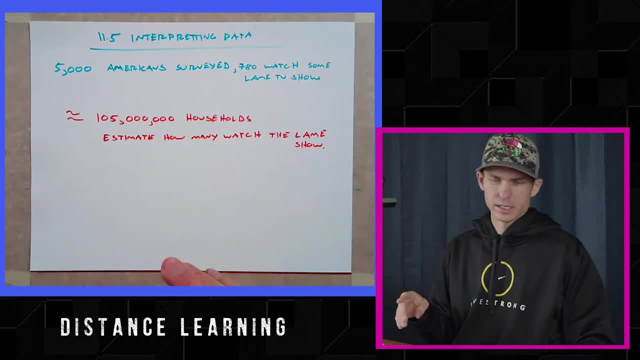 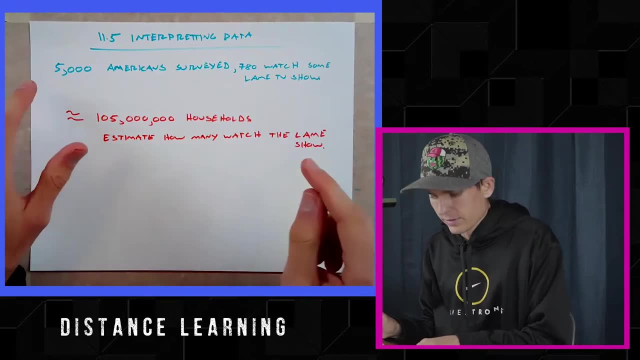 Okay, Okay, Okay, Okay. So you want to kind of use that survey to make a generalization for a larger group of people. So, in this case, 5,000 people we surveyed, which is a lot of people to survey. 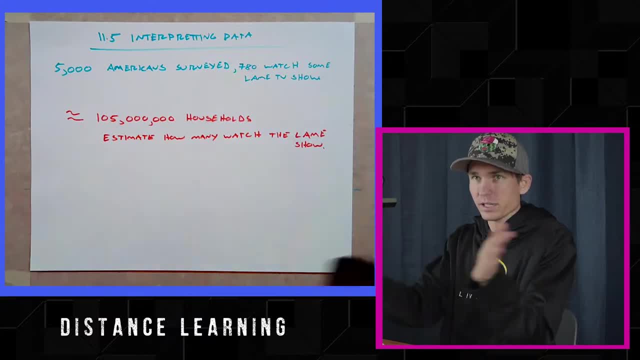 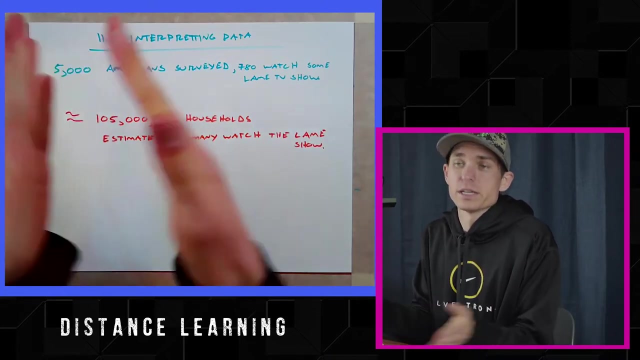 And you want to use that information and you want to kind of generalize that conclusion towards the 105 million people, because it's going to be very difficult to survey 105 million people. So you want to try and use your survey and say this is what I found from my survey, and I think it extends to the rest of the country, for example. 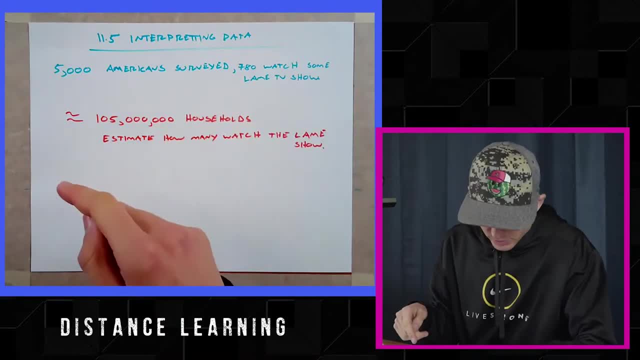 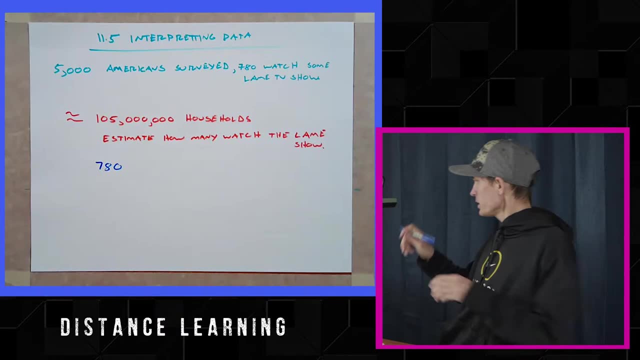 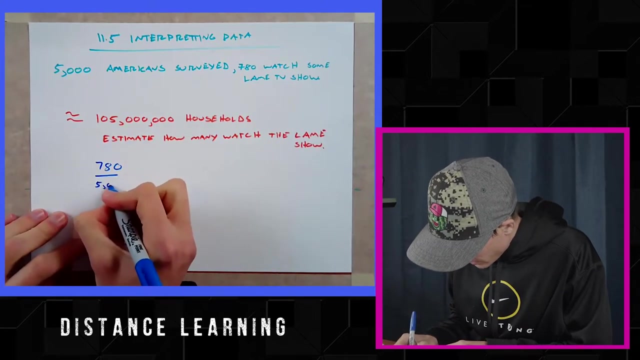 for example. So how many watched the Lame Show? Okay, well, in my survey, right 780.. Oh yo, Mr Hill didn't get a calculator and we know he's bad at math. 780 out of 5,000 watched, right. 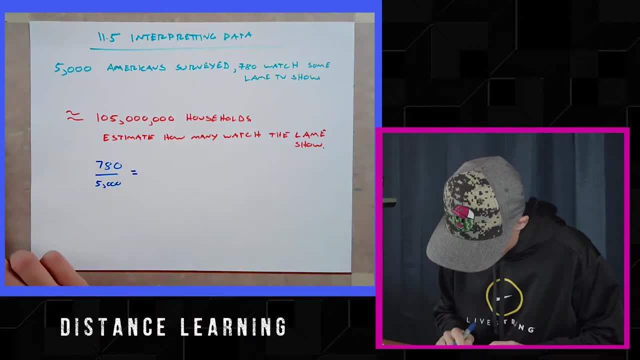 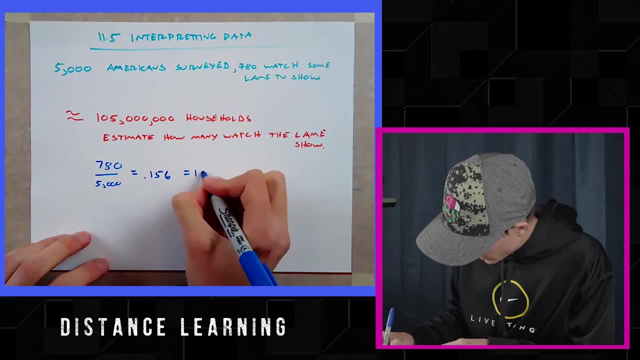 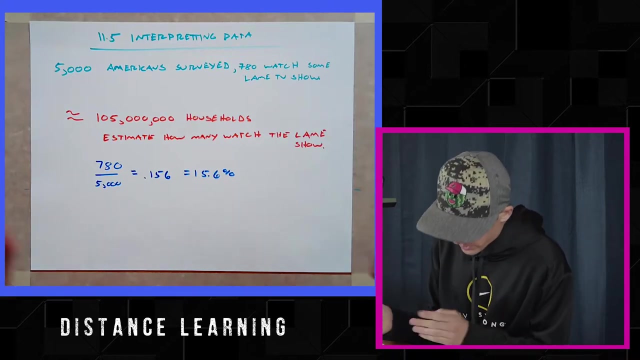 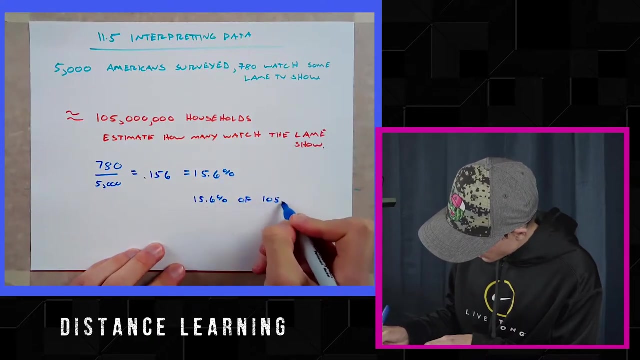 So if you enter that into a calculator and you can't see it in this calculator because the screen's not very bright, that's 0.156, which is 15.6 percent, right? So 15.6 percent watched according to this survey. So then, 15.6 percent of 105 million, right? So you'd. 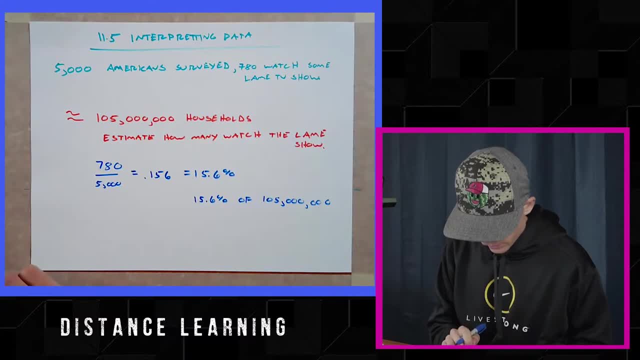 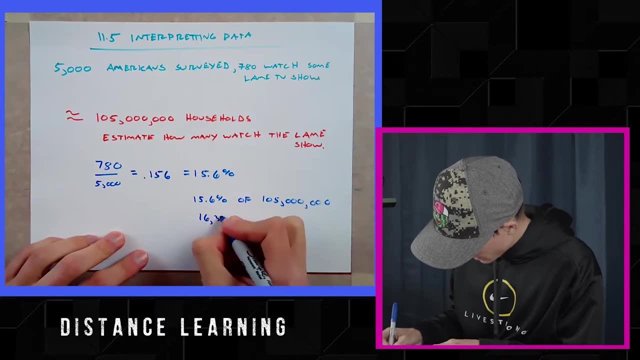 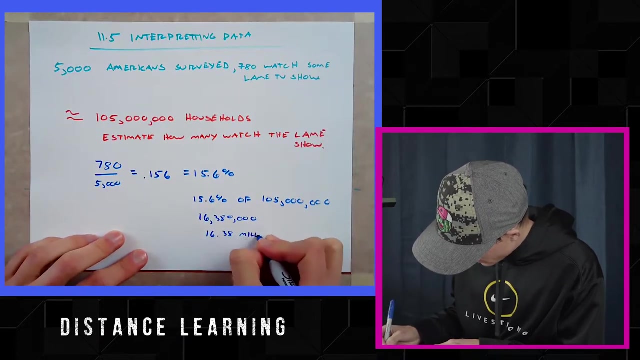 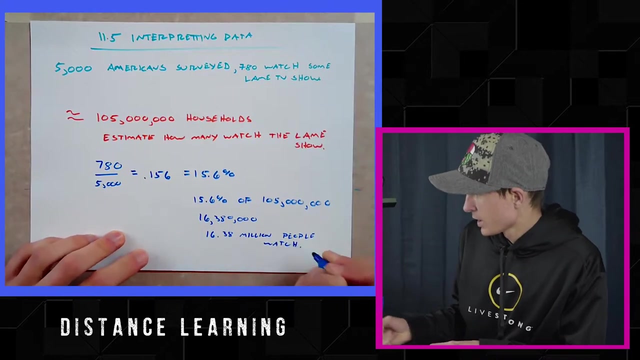 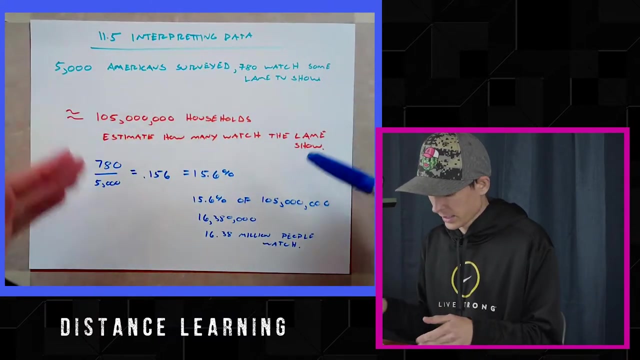 multiply 0.156 times 105 million And you'll find out that 16,380,000 or 16.38 million people watched. All right, and so now your generalization is to the country who interpreted: 5,000 people, survey and extended. 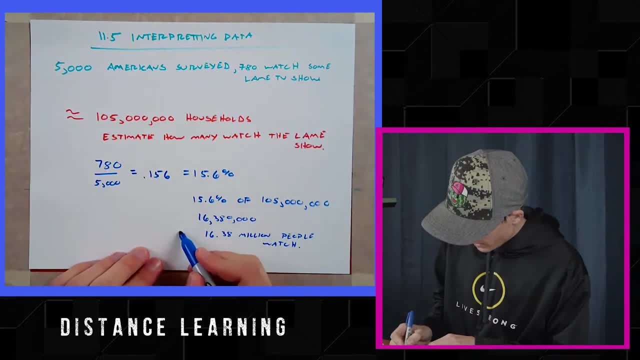 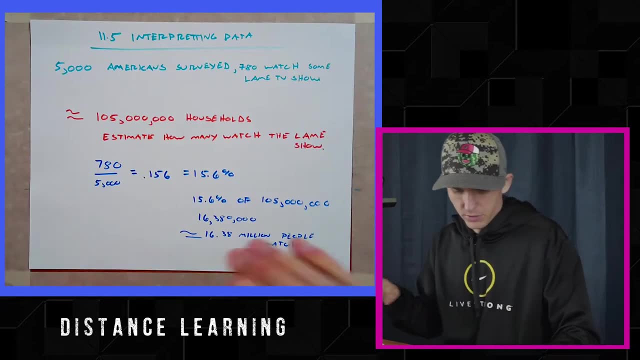 it to the rest of the nation And we found out that 15.6 percent of 105 million people watched. All right, so now your generalization is to about 16.38,. 16.4 million people watched this show. So I surveyed 5,000, but we think that our 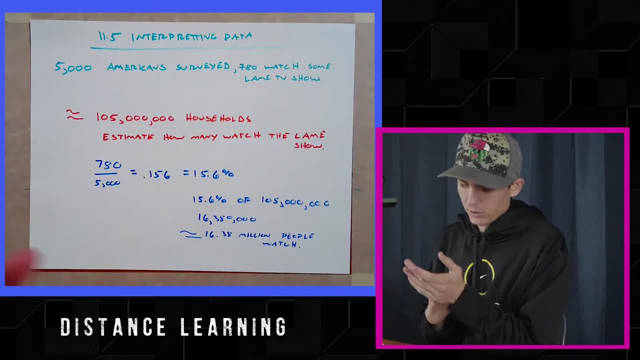 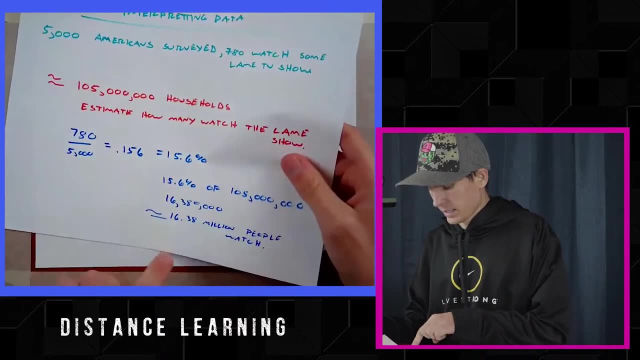 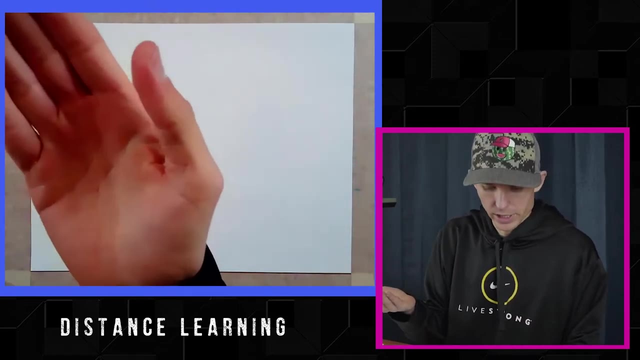 data is good enough to represent more people Now in surveys. right there is. it's probably not exactly that number right, Probably not unlikely. So there's a margin of error. There might be more people who actually watched or there might be less people that watched. 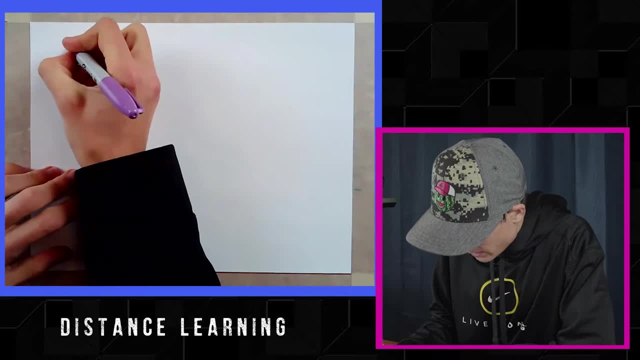 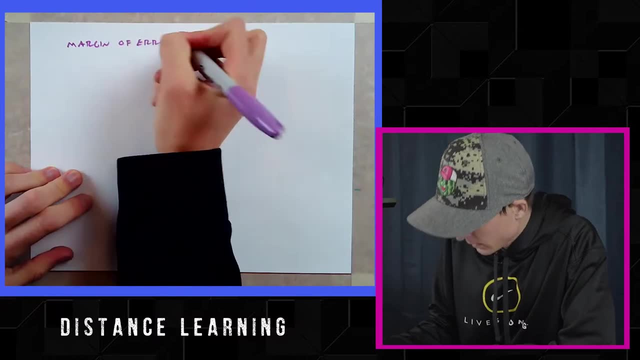 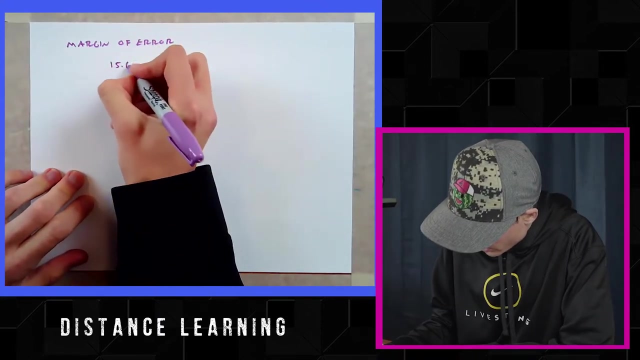 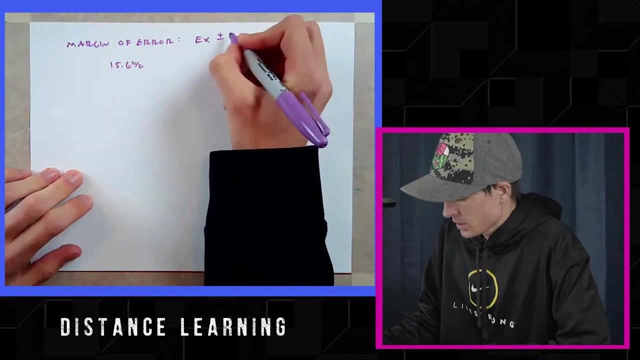 So the kind of buffer range is called the margin of error. So, for example, we just said that was what was it? 15.6 percent is what our survey showed. Example margin of error. you'll generally see it as plus, minus and let's just say three percent. So it could have been, you know. 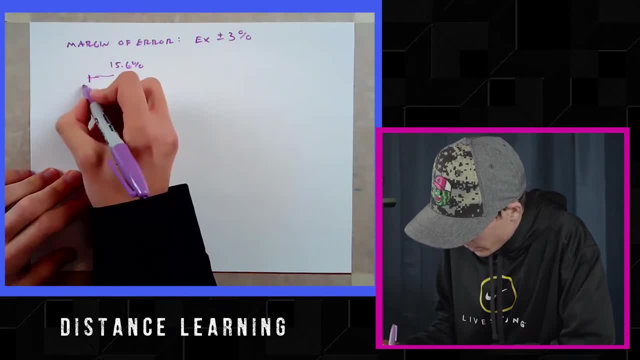 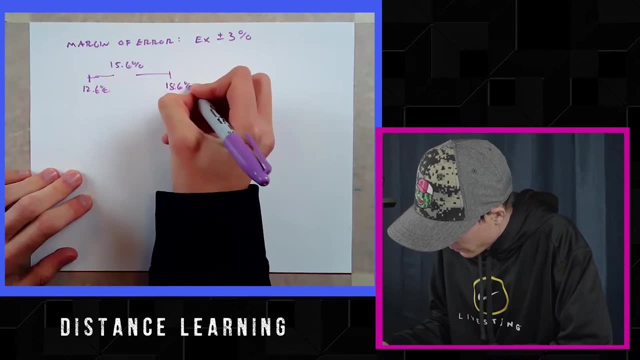 three percent less. So that would have been what? 12.6 percent, or maybe it was actually a little bit more, 18.6 percent. So your margin of error is like: this is what the data shows, but it's. 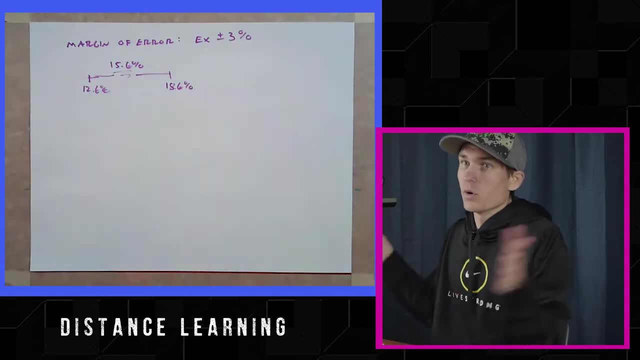 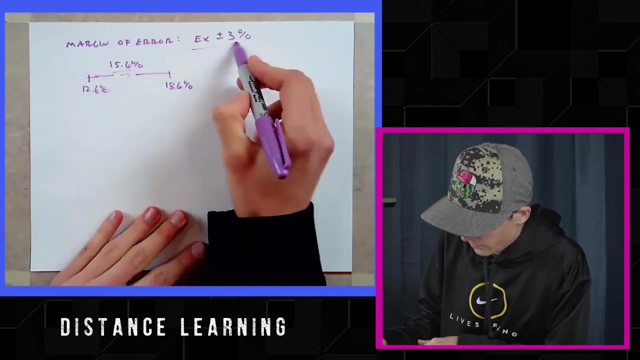 unlikely that it's 100 percent correct if I extend it to more people. So the margin: we're not talking about how to come up with a margin of error. There's lots of math calculations to get the margin of error, but you give it. 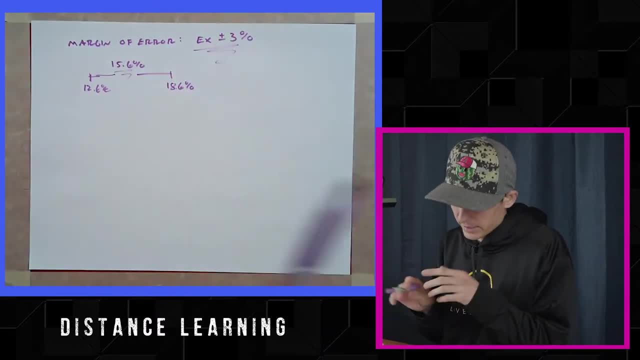 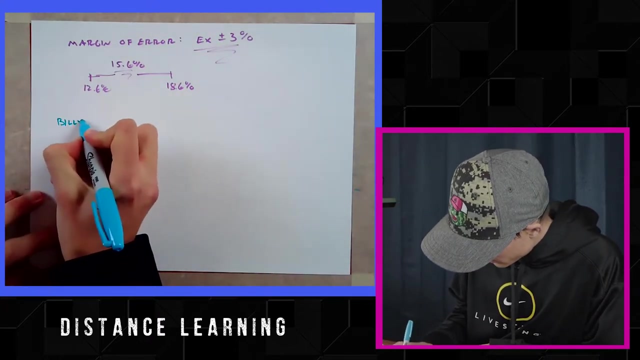 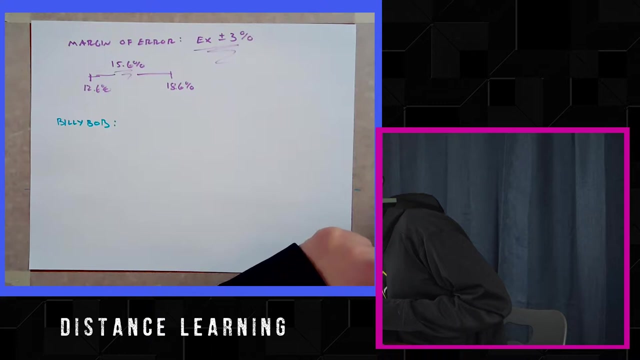 and you're like it might be a little bit less, it might be a little bit more. That's basically the idea behind margin of error. So the classic problem: you're having a election. We got Billy Bob who, according to survey, 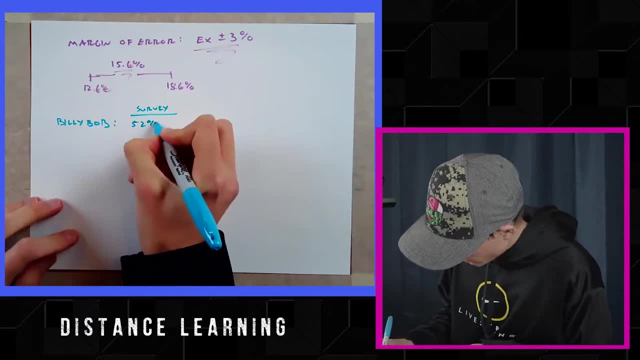 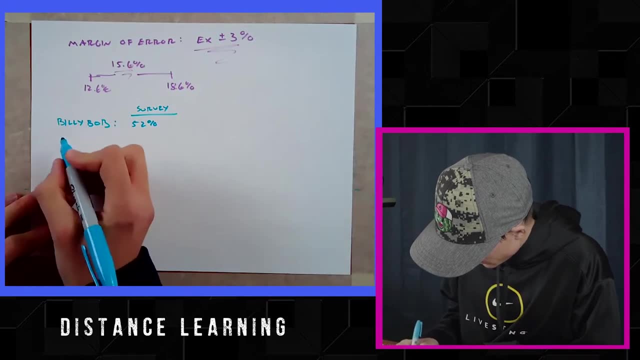 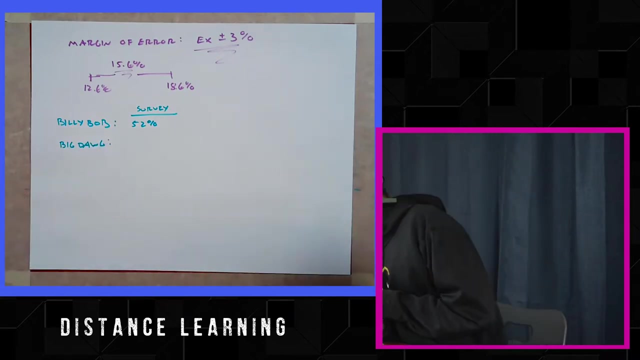 shows that he will get 52 percent of the votes, right. If you get 50 percent, you're going to win. Then you got Big Dog who math dude shows up. he's going to have 48 percent. He's going to lose, right. 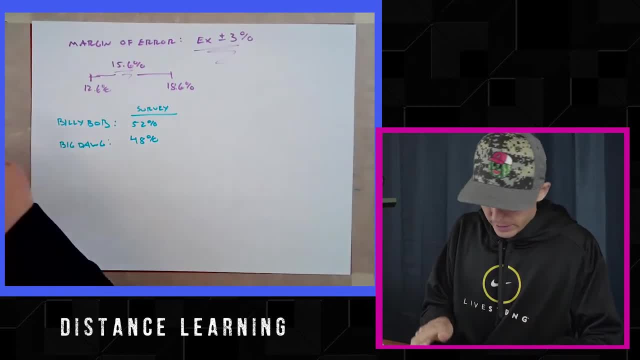 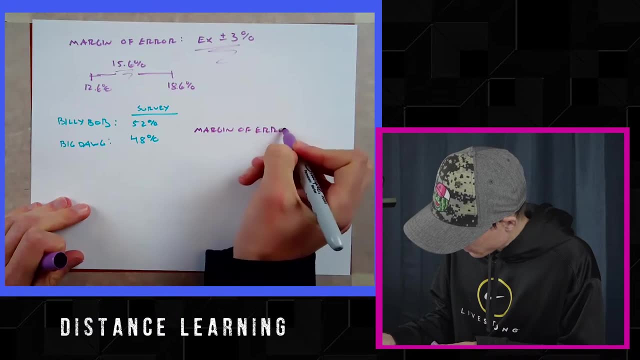 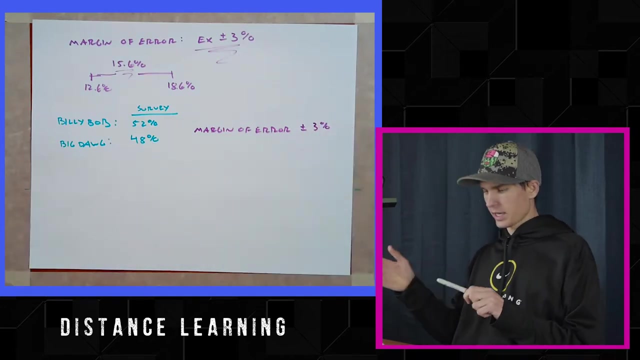 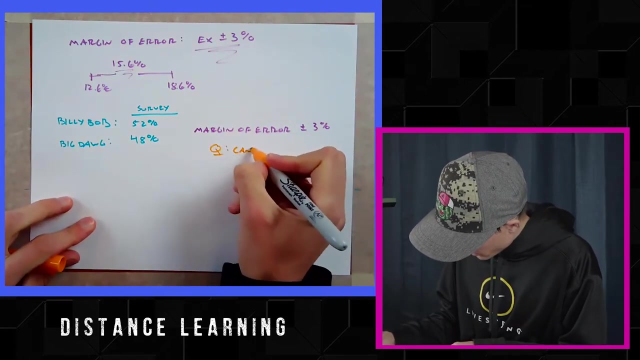 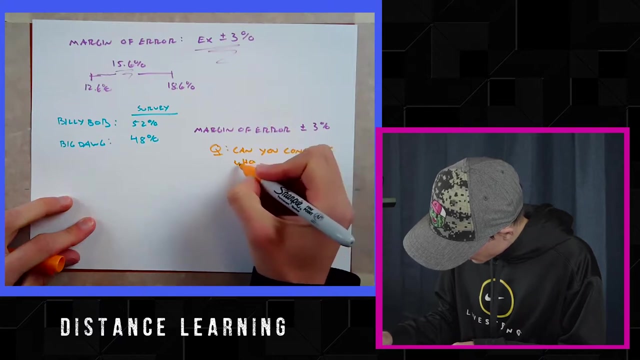 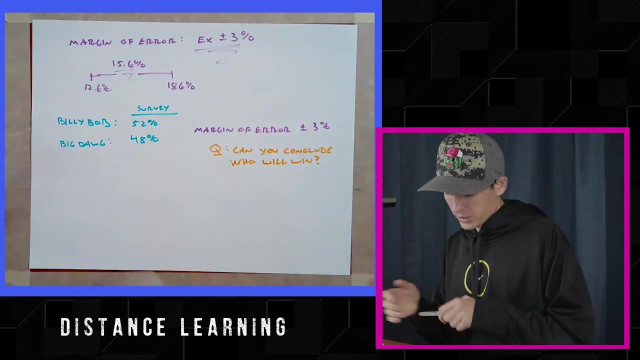 Margin of error. let me go back to that young purple pen. Margin of error is plus minus. ah, again three percent. Okay, The question, can you conclude: who wins? Who will win? So right, it looks like Billy Bob's going to win over Big Dog, right, However, with the margin of error. 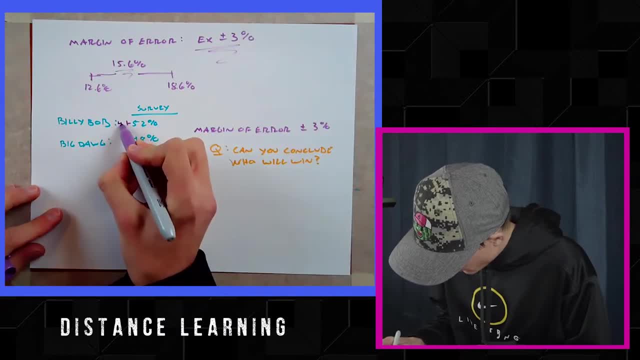 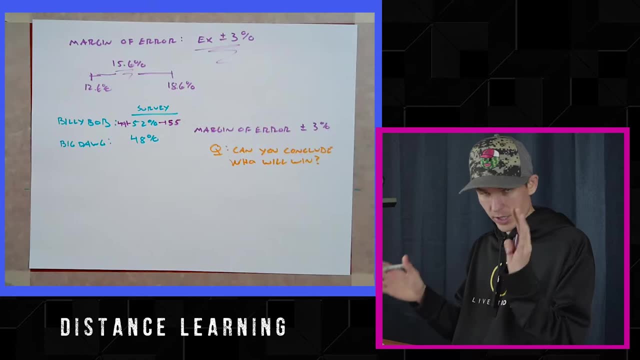 if you subtract three he's going to have 49. If you add three he could have 55 percent right. So he's in the range of 49 to 55. And if you subtract three here Big Dog might only get 45,. 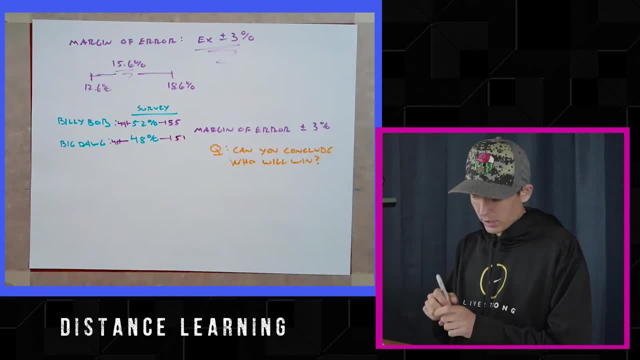 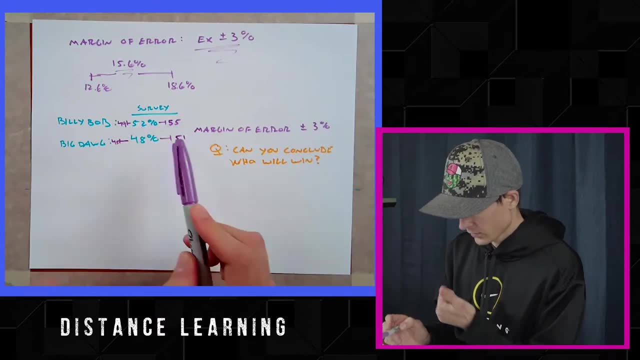 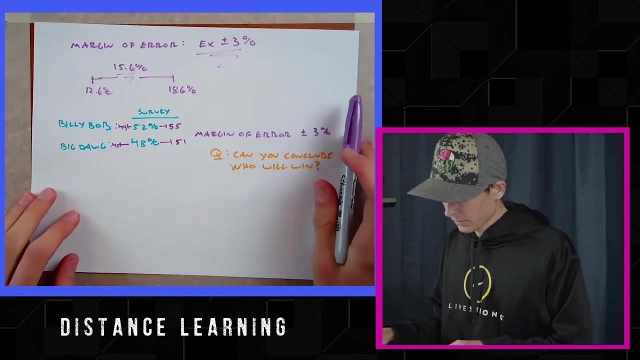 or he might actually get 51.. so, while it looks like there's a larger chance- right, because there's more above 50, right, he only has 50- 51, but this dude has 50, 51, 52, 53, 54, 55 more numbers above 50, 50 or above than big dog. 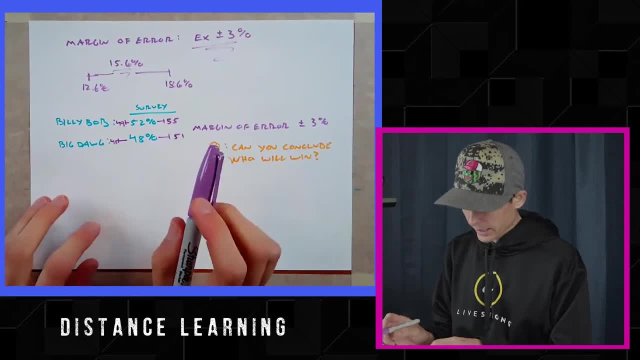 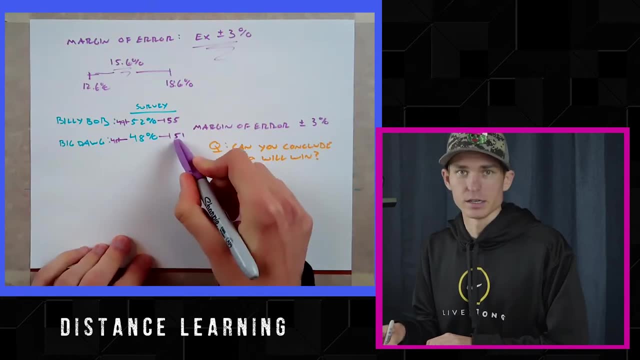 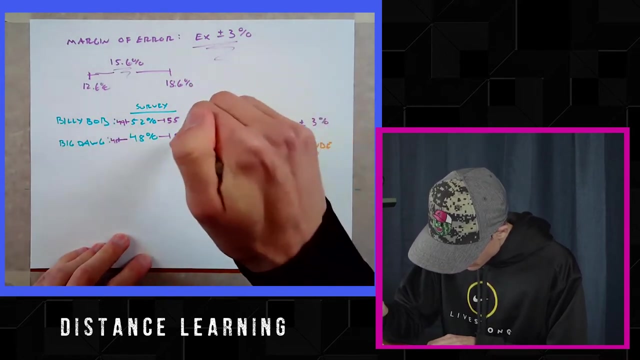 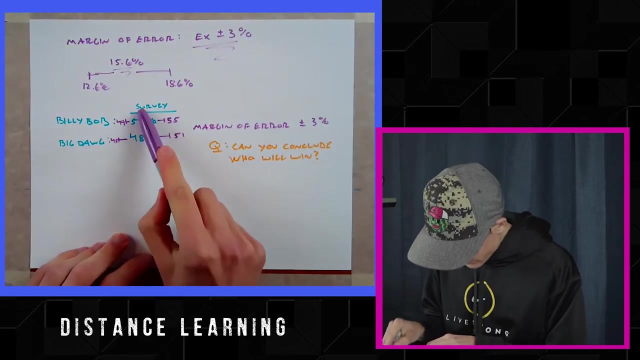 does right. so it looks like billy bob will probably win. however, based on the data and the margin of error, there is a chance that big dog will get 51 and billy bob will get 49. so in the data i can see explicitly 51- 49. big dog could still win if these results are actually true: 52, 48. 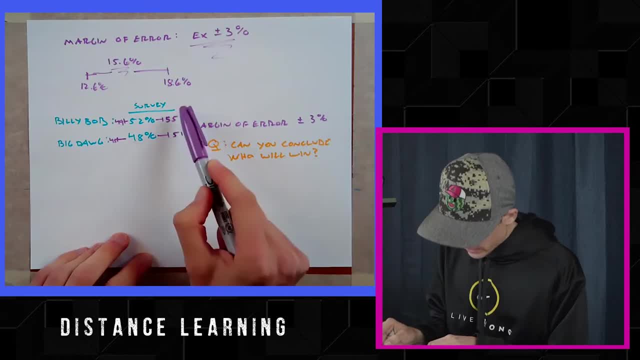 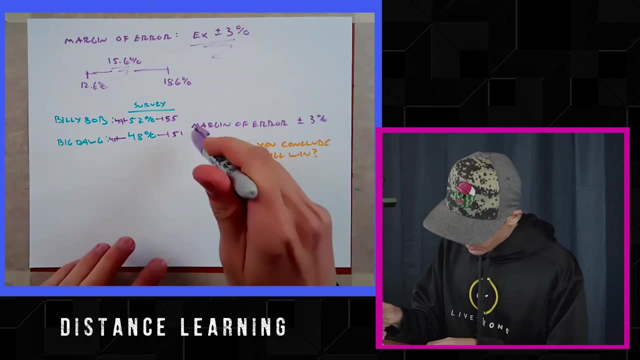 billy bob will win right. or if you got the higher end 55 and big dog got 45, uh, billy bob also wins you. however, there's still the chance that big dog gets 51 and billy bob gets 49. so you cannot conclude. 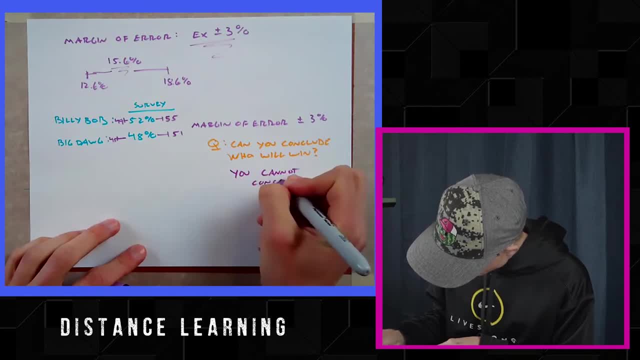 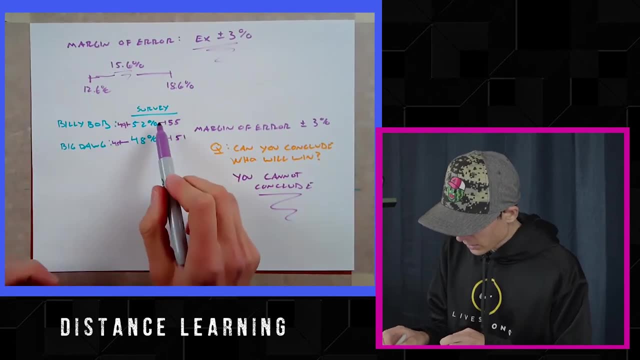 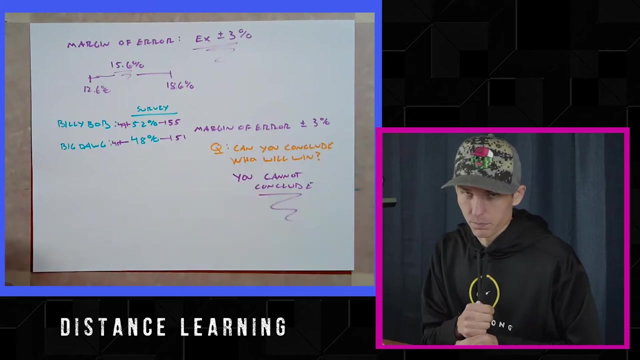 who will win? okay, now there's any of everything in between. it could be like 50, 50, it could be 53, 47. anything in those ranges that they give us based on the margin of error, are possible results. okay, so hopefully that's synced in with you guys. 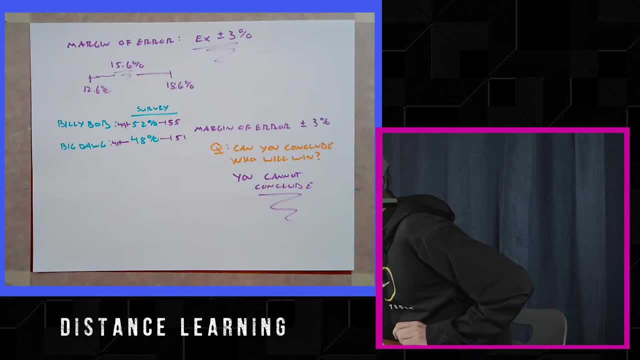 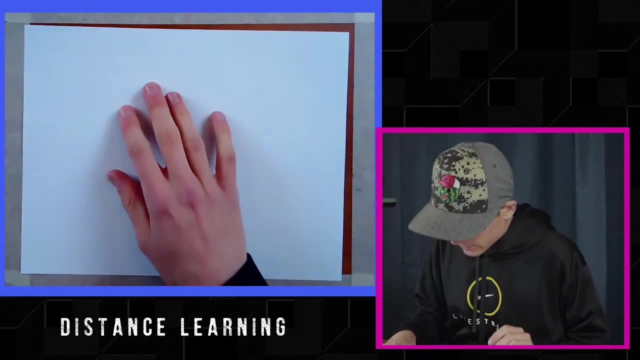 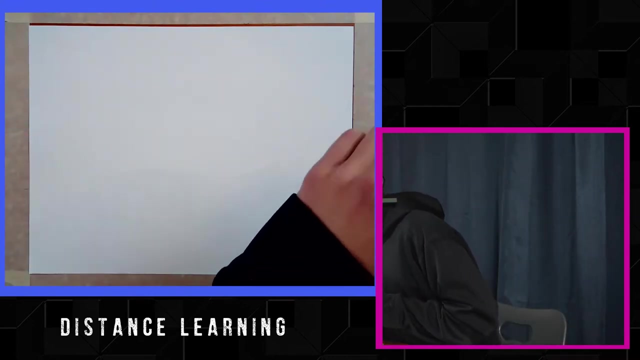 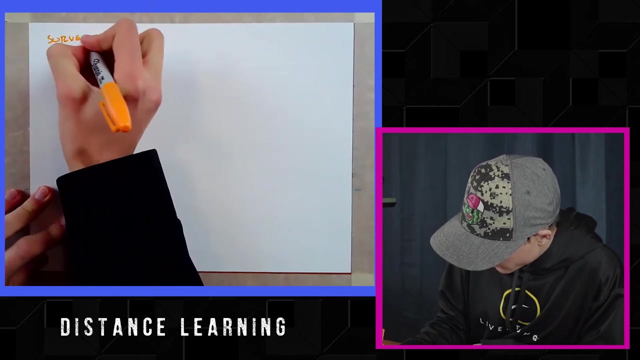 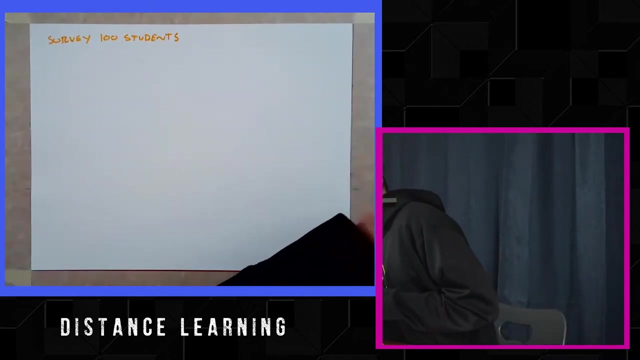 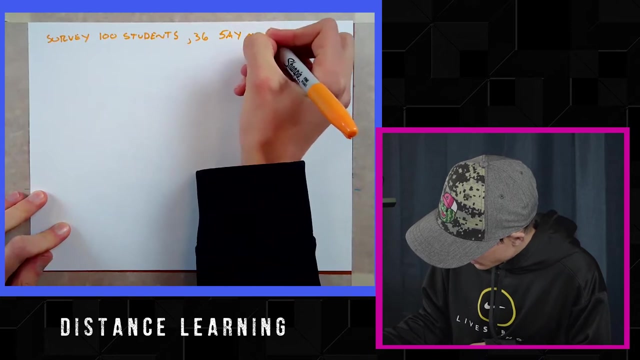 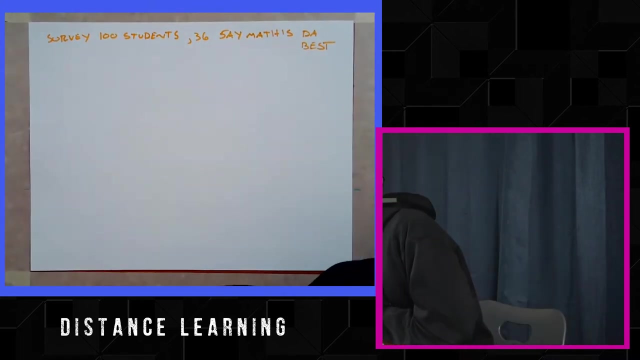 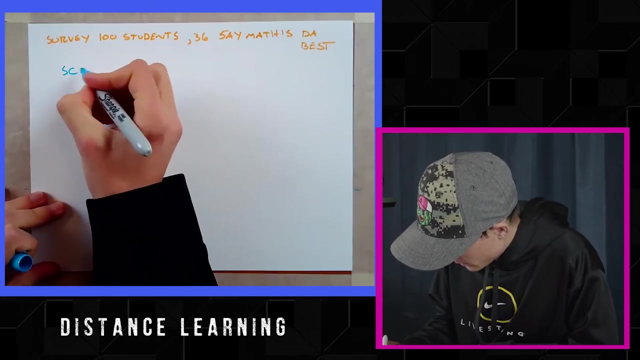 i'm gonna skip that. y'all can read that example. whatever i write, i'll do number six, number six, number six. favorite subject: obviously not math. so you survey 100 students, 36 say math is the best. it's a big school though. the school has 1200 students. 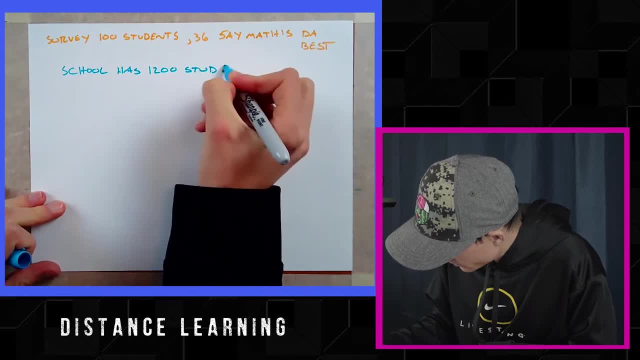 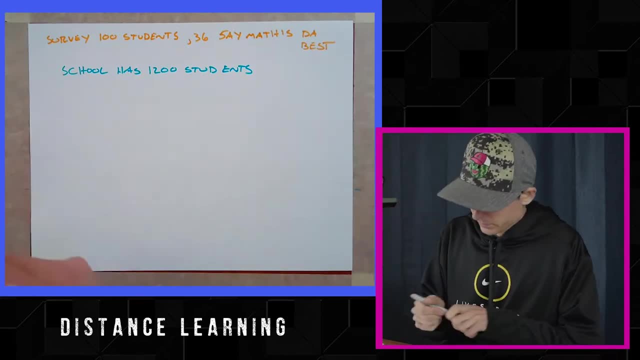 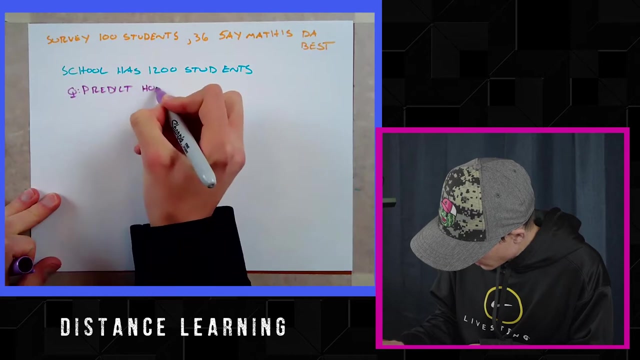 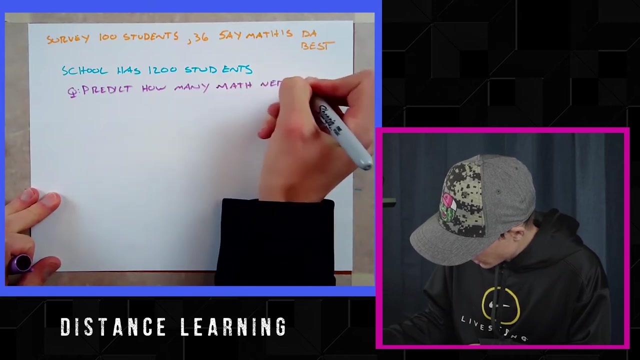 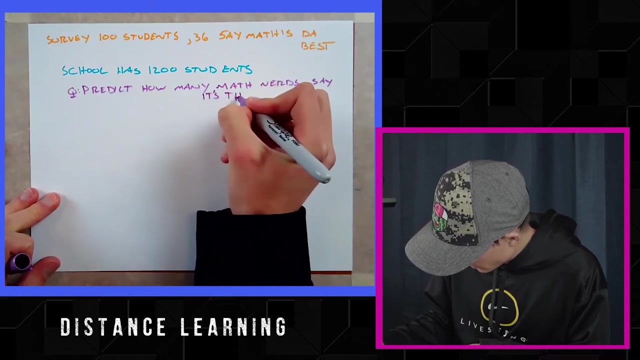 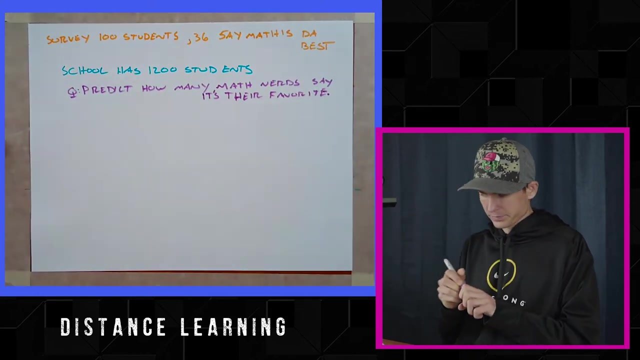 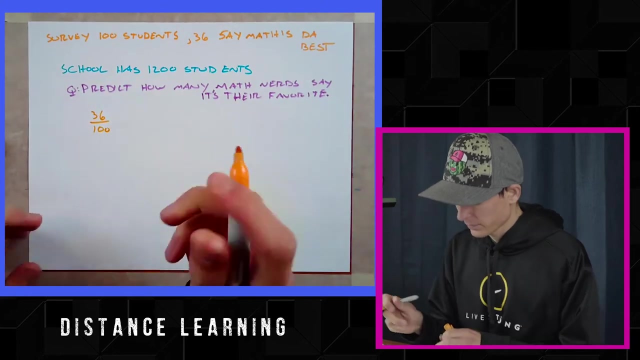 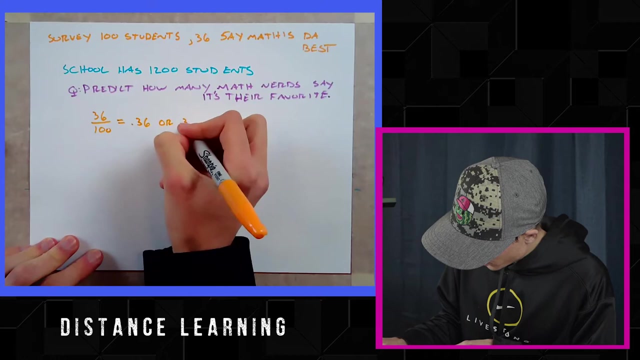 the school has 1200 students. the school has 1200 students. right, predict how many would say math is their favorite question. predict how many math nerds say it's it's, it's great. math is their favorite. the math jar, it's good. okay, so it's gonna reveal adulthood. 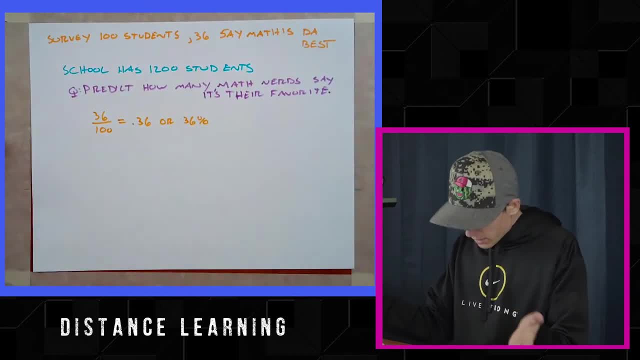 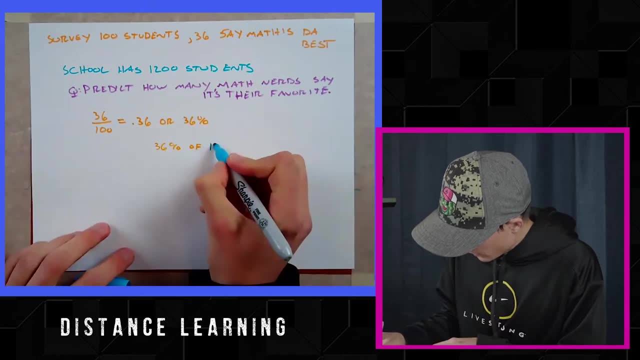 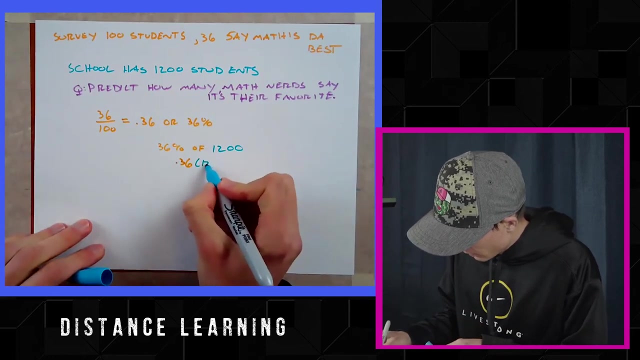 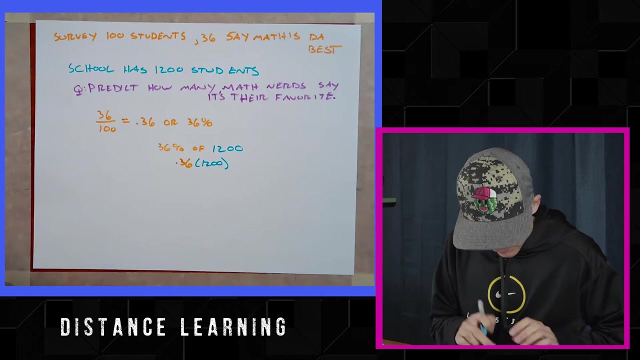 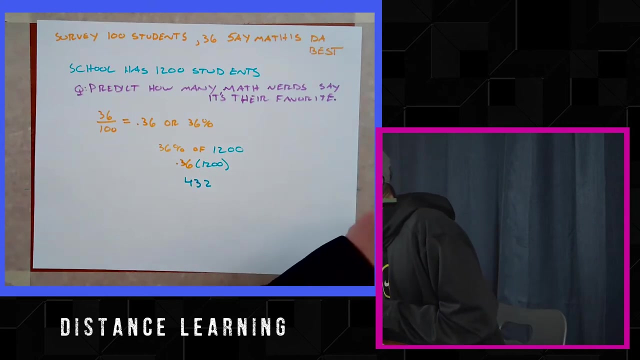 students have. they need to be nervous, they need to be afraid of the sun, for sure of 1200. so I'm going to do 0.36 times 1200 and I'm going to get 432. what did I do? really bad math. I think the book is way off on that one. the book says 360. I don't think so. 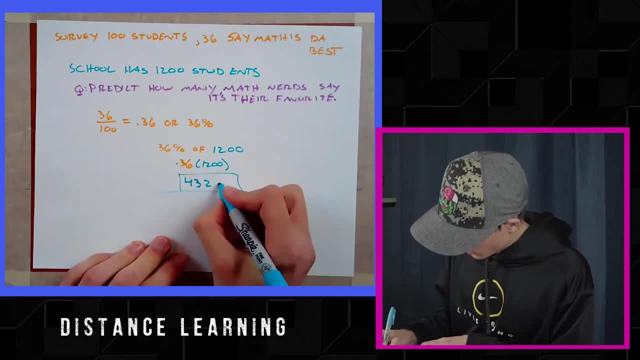 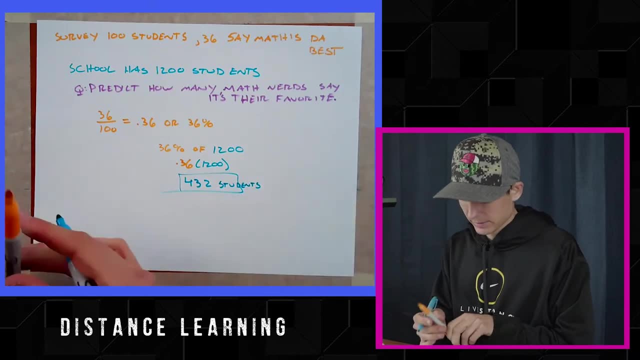 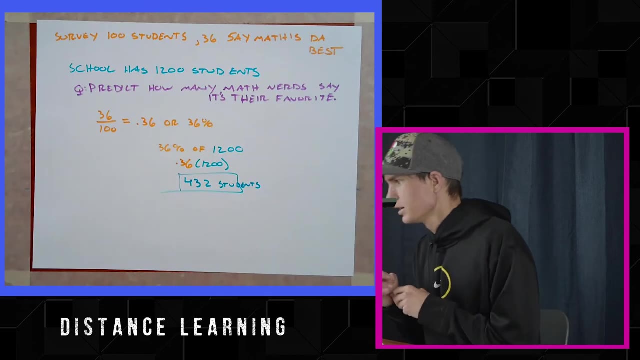 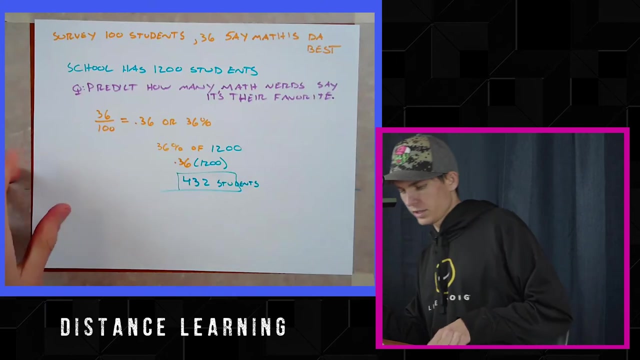 yeah, that's not right. about 432 students would say math is their favorite subject. so it's at 36 percent, 36 out of 100, and then you extend that towards 1200 total students. I know what they did, but they're not doing that good. so, number eight, you've got this book. 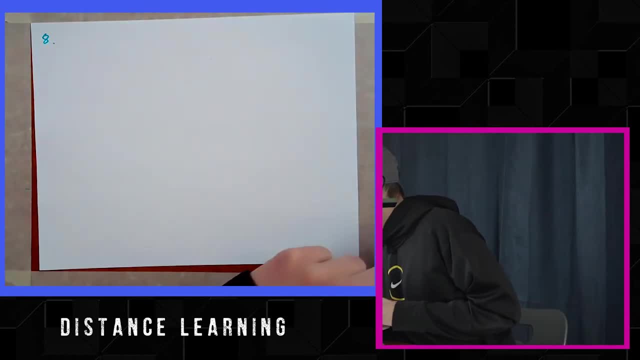 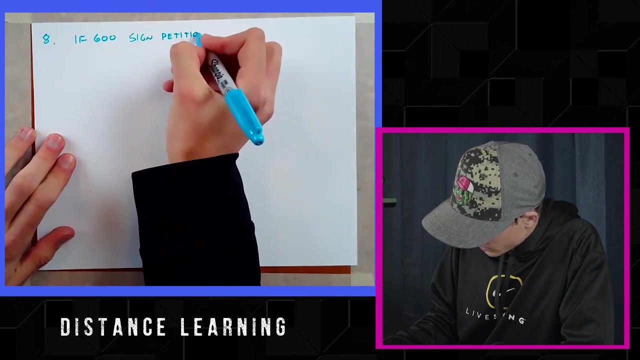 so well, there might be five or 16 books. do you guys have a $2.30 end customer here? do you guys know a book about? Wasn't that a very good one? I know that's right. yeah, that was one doing that last one. oh, that's good. 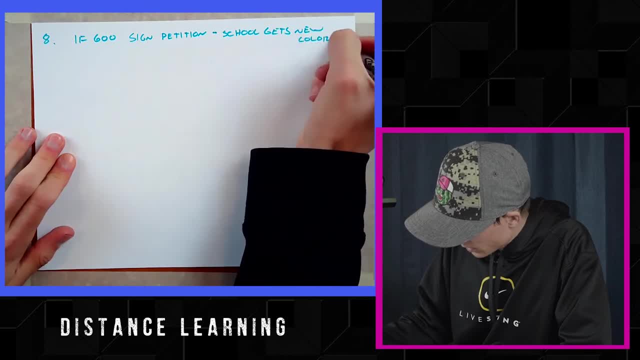 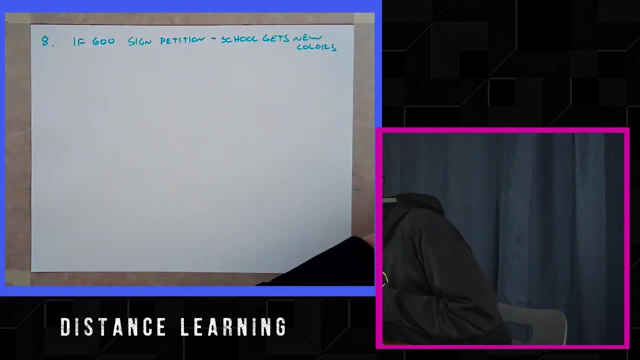 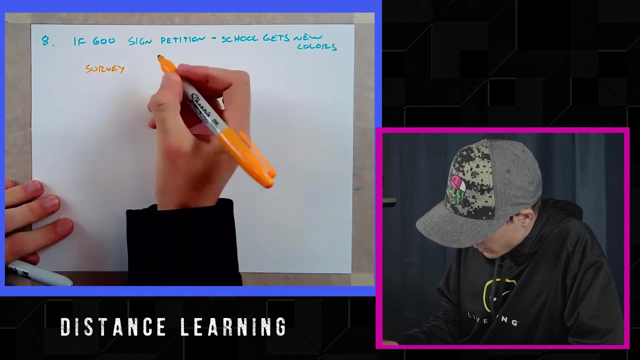 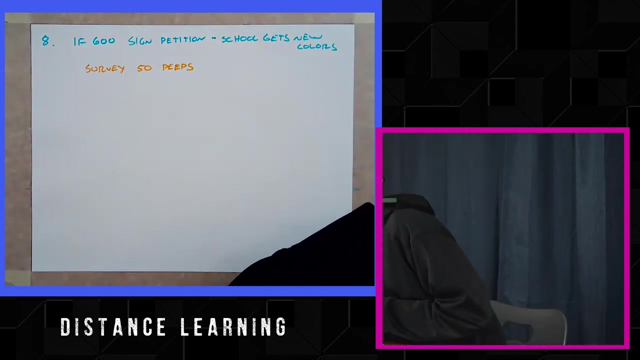 and then this says: a school student council said it would change the school's color if 600 sign petition. school gets new colors, school gets want a new uniform. all right, you interview a random sample, you survey 50 peeps short for people and 37 sign your petition, right. 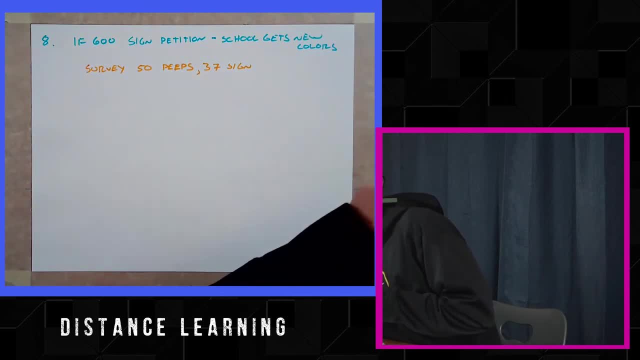 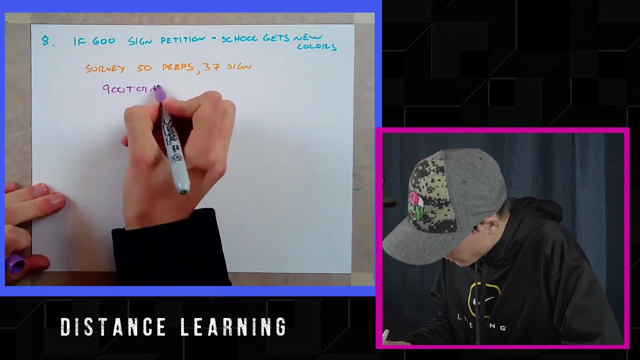 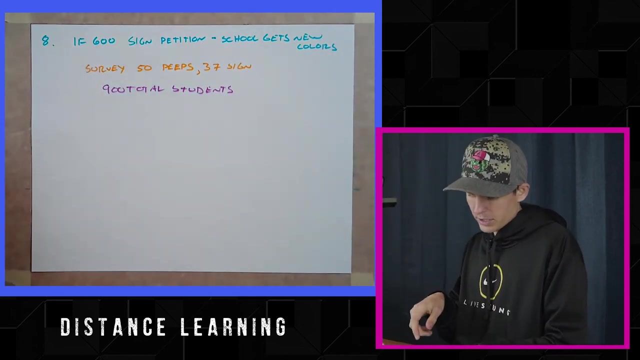 school has 900 students- 900 total students in the school. do you get enough votes based on your survey that you're gonna be able to do this? so right, I need 600 signatures. I'm gonna go up to probably more than 600 people to get my votes right to change the school colors. 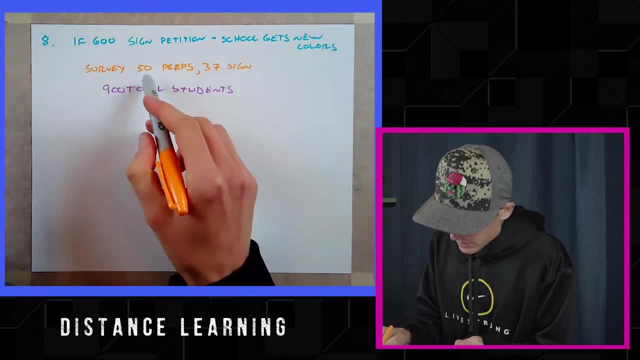 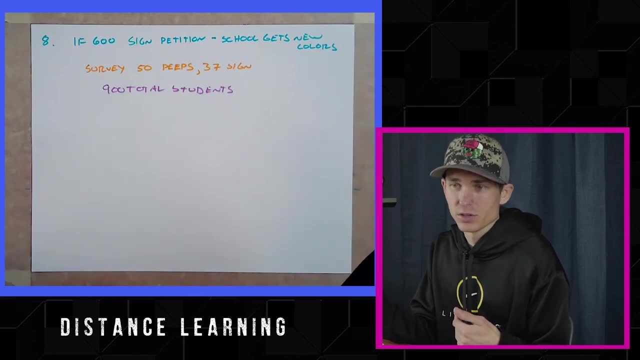 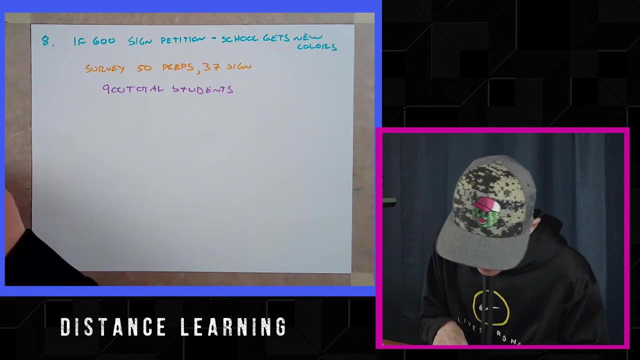 I'm gonna say I'm gonna do 50 people and see, based on that data, is this really gonna work out and I should keep doing this, or am I really like: ooh, I only got like a few people to sign out of 50. there's no way I'm gonna get 600, so I'm gonna stop wasting my time there, kind of. 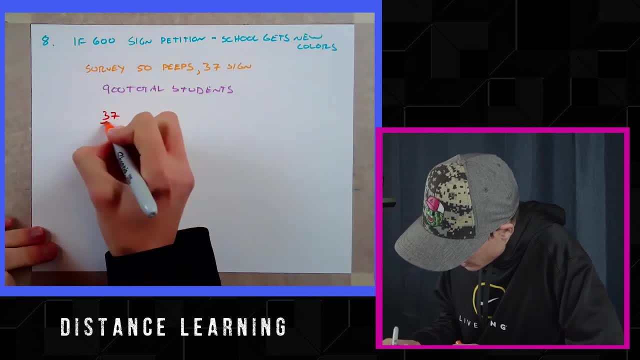 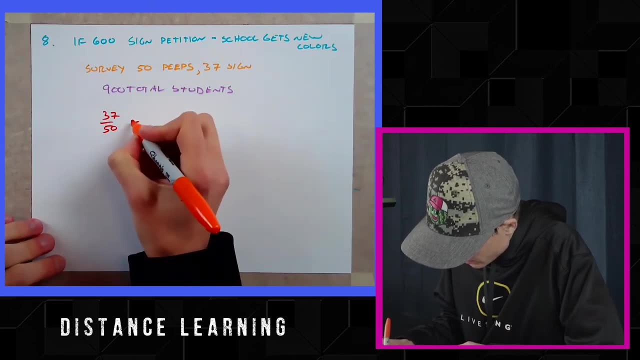 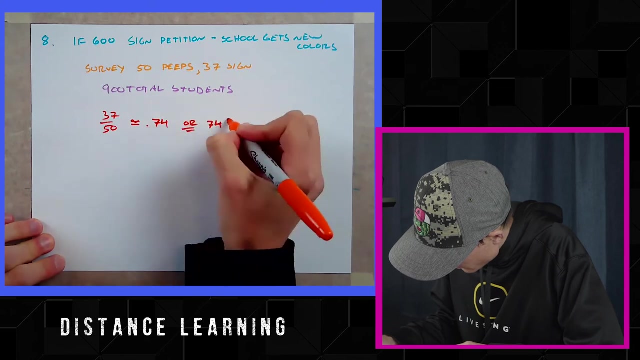 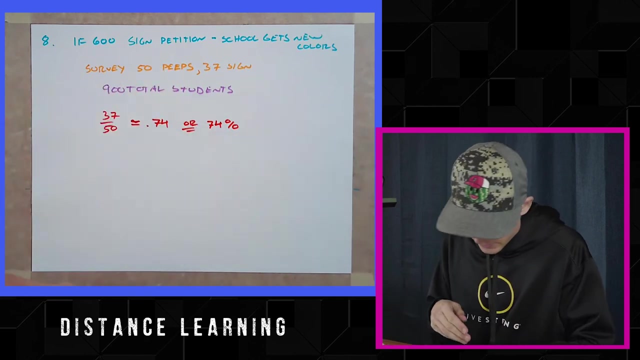 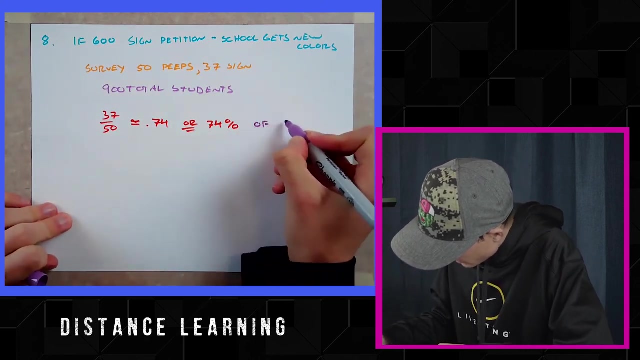 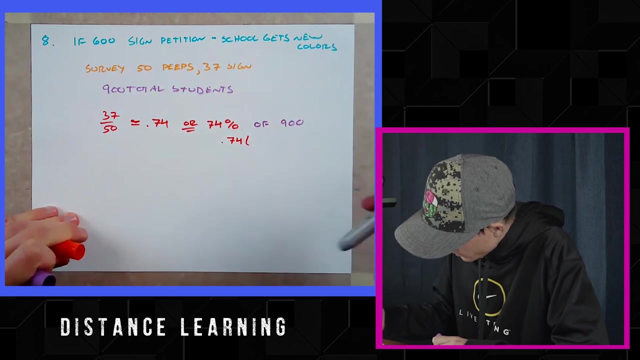 thing right. so my 37 out of 50 right, that's an easy one- is not about equals 74%, okay, I'm like that's pretty good, that's pretty good, that's a nice number. so I did 50 people right. so if I did 74% of 900 right, that'd be point seven, four times nine hundred. 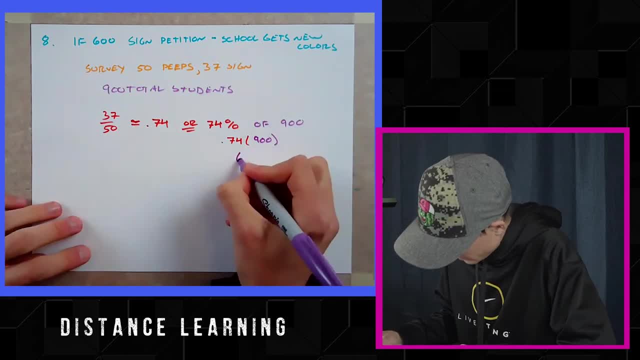 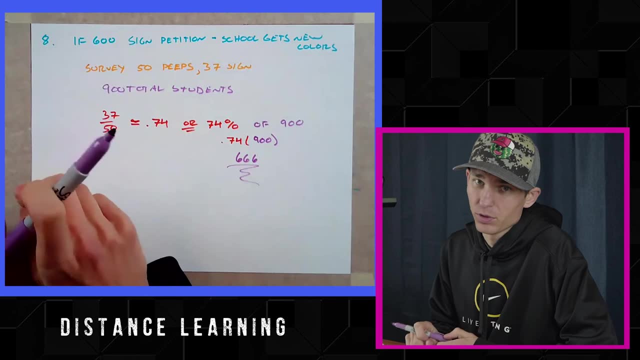 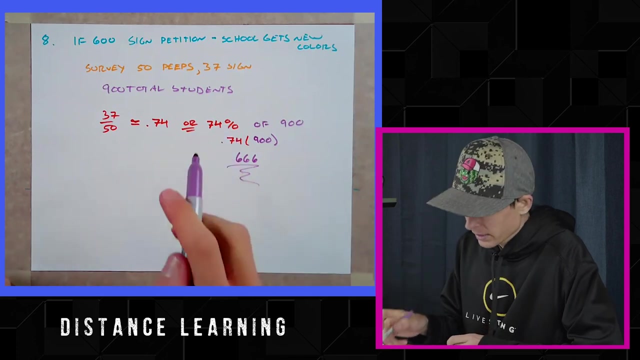 oh, not a nice number, definitely number. I get 666 and I see like that's 66 more people than I need. so even if I get a little bit less, I think, I think I can put in the work and I'll be able to get the. 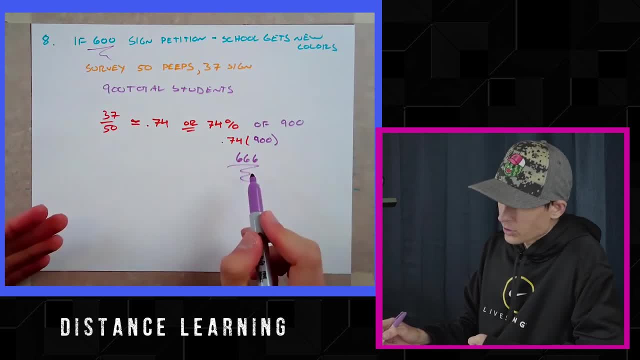 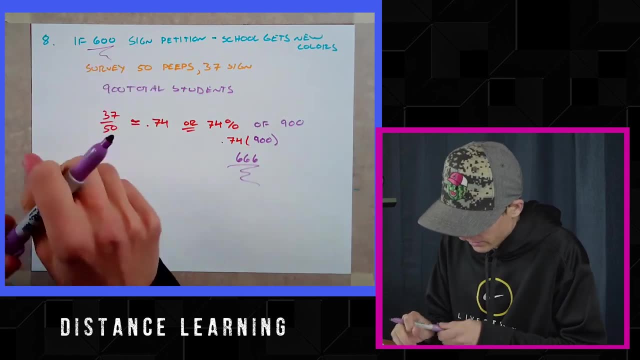 result I want. if I found this percentage- I got like 500- I'd be like, hmm, it's not looking like even if I keep doing this, I'm gonna get my 600 people, because it's obviously not that popular of an idea. however, your data shows that you think you'll be able to.